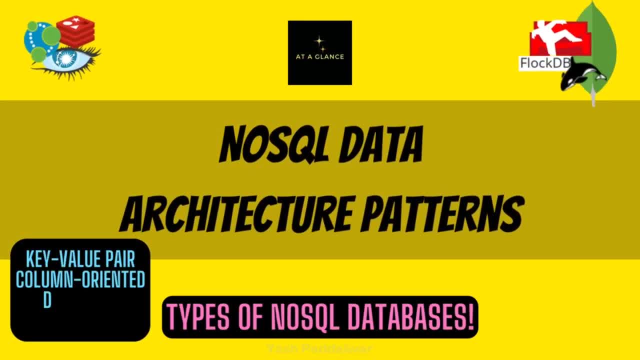 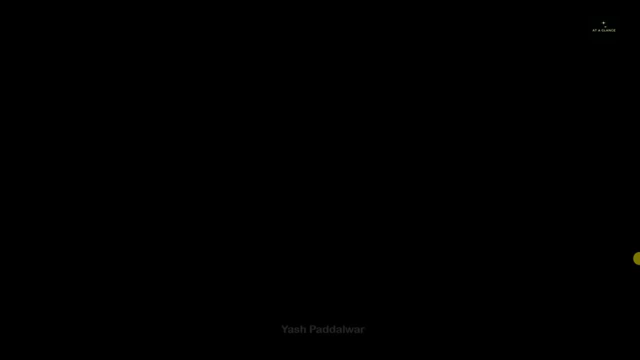 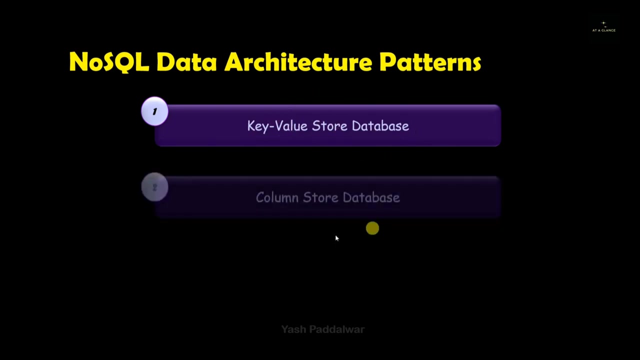 Hello everyone, welcome back to my YouTube channel. In the previous video we have seen NoSQL introduction and we also have seen the CAP theorem. Now it's time to look into the different types of NoSQL databases. That is nothing but NoSQL data architecture patterns. 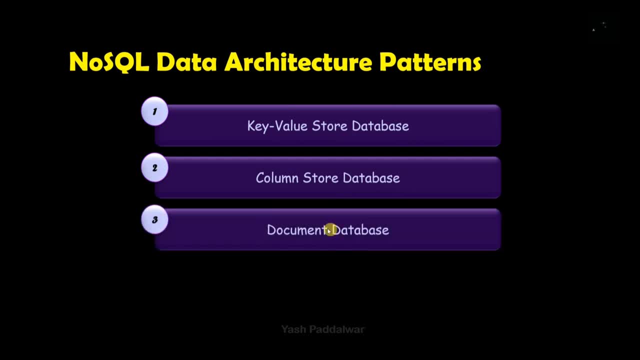 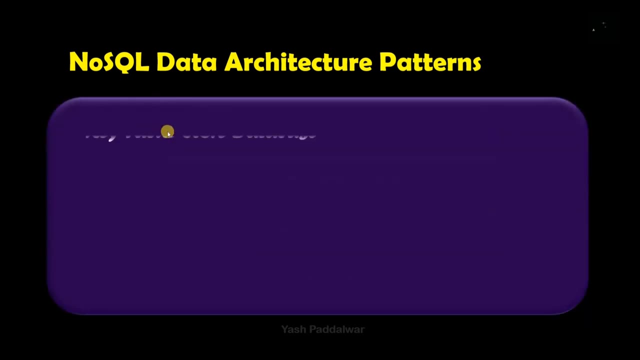 So total, there are four NoSQL data architecture patterns. First is the key value store database, Next we have the column store database, Next, document database and lastly, we have graph database. All these databases are very much important when it comes to NoSQL. Let's start. 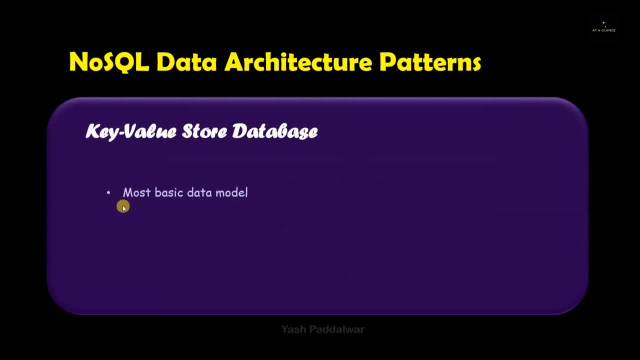 looking into detail in all of them, one by one, starting with key value store database. So this is the most basic data model of NoSQL. As the name suggests, it stores the data in the form of key value pairs. Now, what is this key? Key is nothing but a representative. 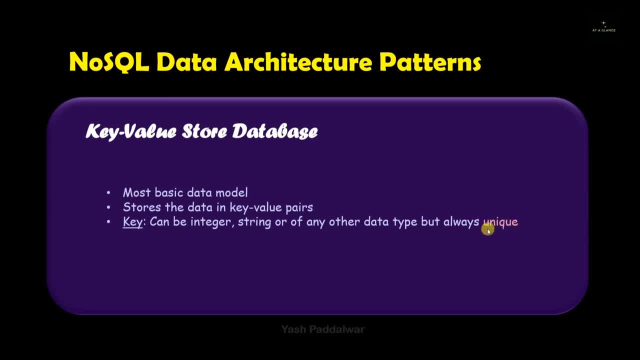 of a particular data value. Now, this key can be any integer string or it can be of any other data type, but it must always be unique because this key is going to be uniquely identify the data that is stored inside it. Hence, key has to be unique. Now, value is nothing. 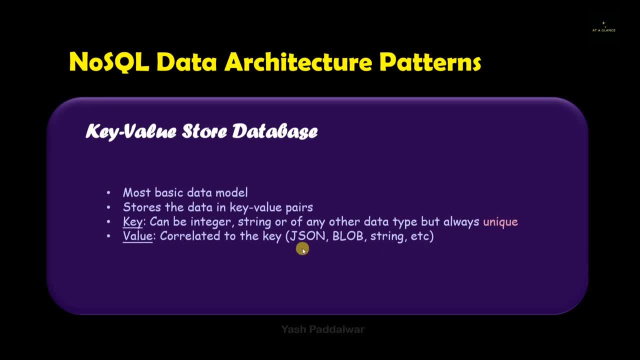 but a data which is correlated with the data that is stored inside it. Now, value is nothing but a data which is related to the key. It can be of the form JSON, which is JavaScript object notation, or it can be block, which is binary large object. It can also be in: 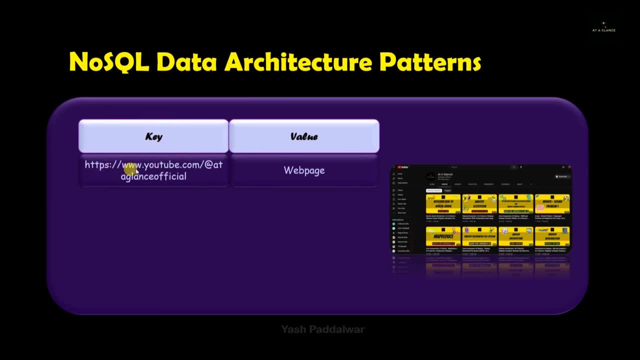 the form of any other data structure. Now let's see an example. Here you can see, the key is a web URL. Here the URL is acting as a representative to the entire web page which is present before it. Hence, URL is the key and the value is the web page which is present. 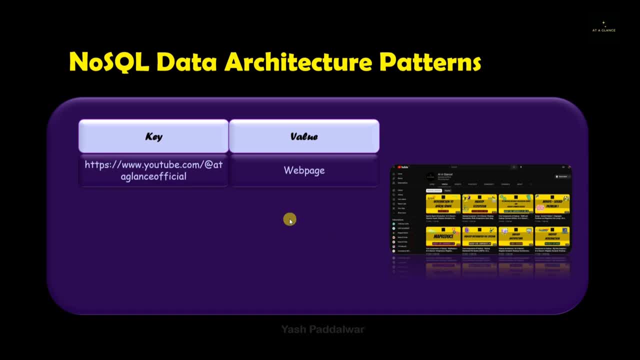 in that URL. So this is an example of the key value pair data. Next example is the name of the file. For example, we have at a glance, logo dot jpg. This name is representative of the file present inside it, and note that name of the file will always be unique in. 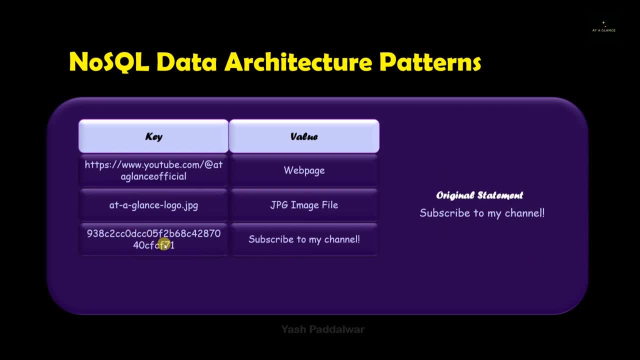 a particular directory. Hence the name is the key and the file which is present inside it is the value. Similarly, we can have the key as the MDFI hash, which is nothing but a hash value that is generated for this particular value. statement that is subscribed to my channel. 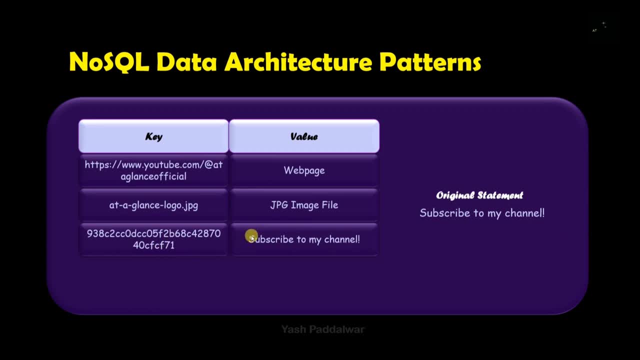 So this hash value acts as a key and the original statement acts as a value. So I hope this is clear. Let's see one more example. Here we have directory path to a particular file, which is patterns dot PDF. So the key is the particular path and the value is the entire. 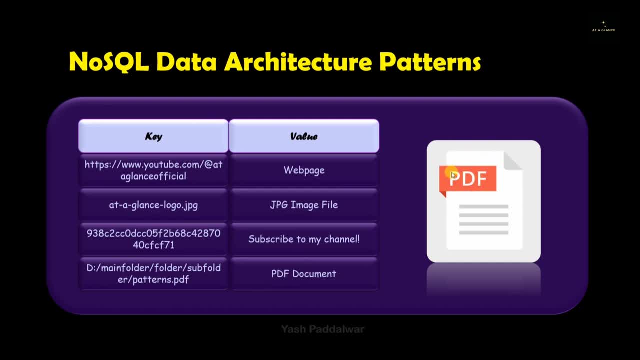 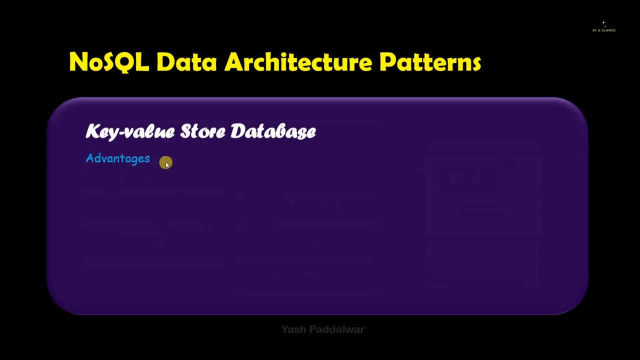 file which is present in that particular path, which is nothing but patterns dot PDF. So I hope this entire key value pair concept is clear to you all. Now that we have seen the entire overview and example of the key value store database. Now let's see the advantages and disadvantages of it. The major advantage of this key value: 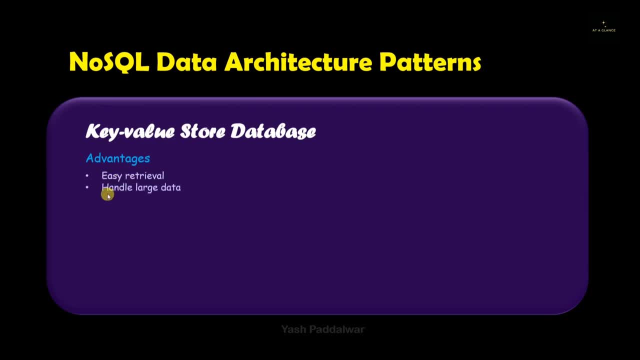 store database is that it can result in the easy retrieval of data, because this is the most basic data model. Its complexities are less, Hence it can handle large amount of data. But the disadvantage is that it has low performance And when complex relationships arise between 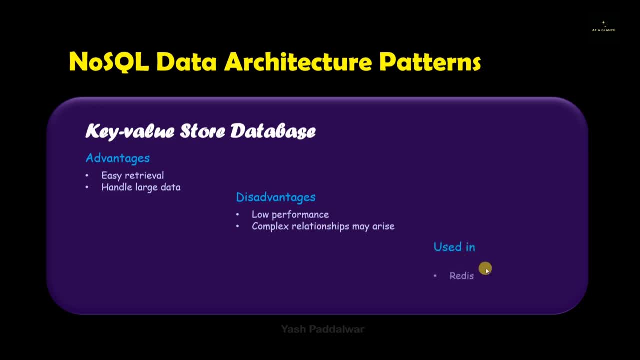 some key value pair, then it can slower the response time. Now this key value store concept is used widely in databases like Redis and React, So I hope this entire concept of key value store database is clear to you all. If you get any doubt, post it in the comment. 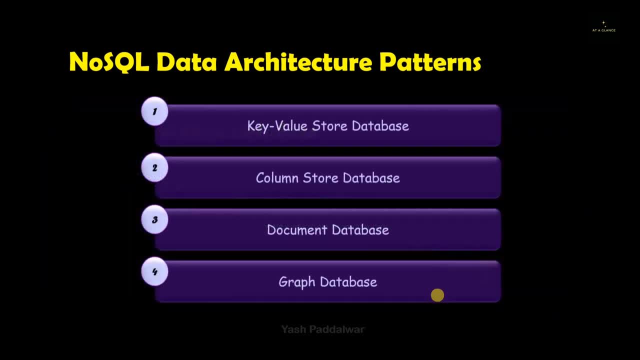 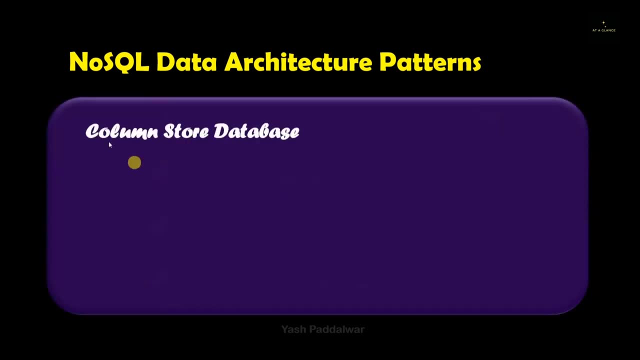 section. Now let's move on to another type of data architecture pattern of NoSQL, which is the column store database. So let's have an overview of it. So in column store database the data storage is done in individual cells. You can relate: 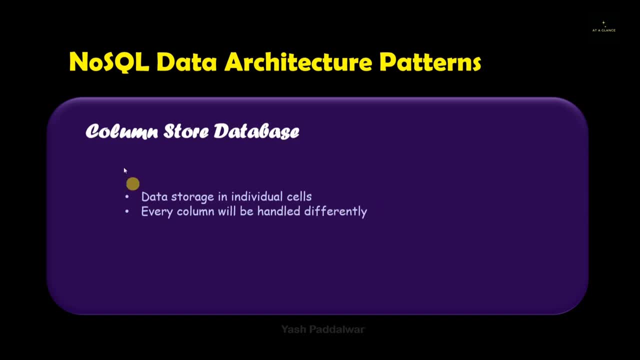 this with your RDBMS. Here every column will be handled differently because all the columns coming under a particular column will be handled differently. So in column store database every individual column is functioning separately. You can note one thing: that individual column will contain several columns inside it. Let's have a look at a simple example to understand. 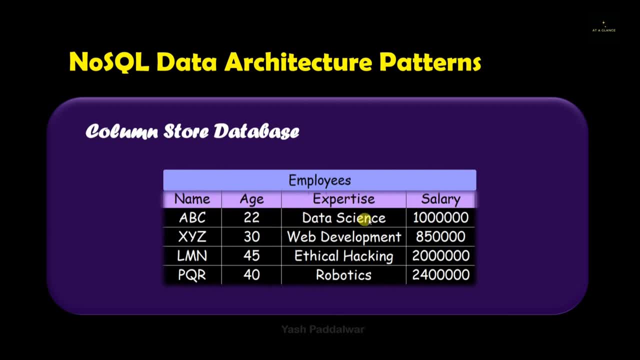 this concept. So here you can see, there are certain columns- name, age, expertise, salary- And on top of this there is a single column which is employee. So we can clearly come to know that all these columns name, age, expertise and salaries. 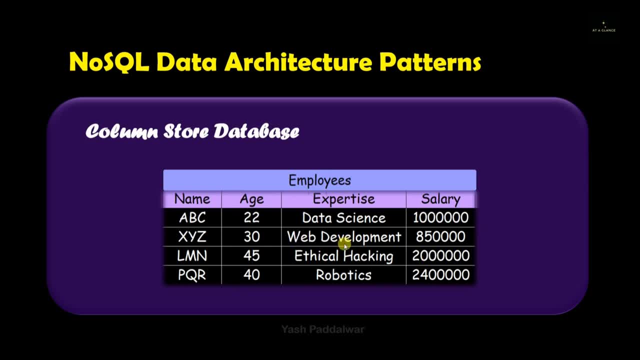 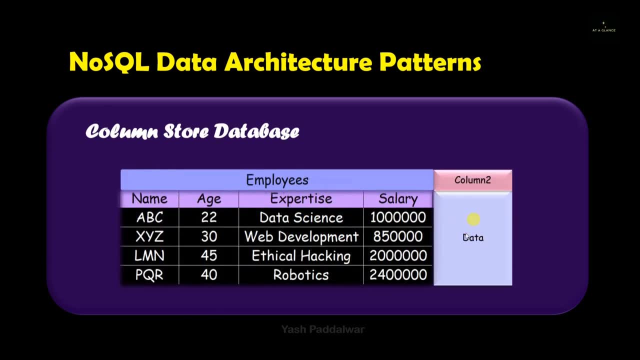 are the data of all the employees inside that company. Hence employees is the super column, and name, age, expertise, salary are all the columns. Similarly, we can have some other columns. For example, at the right of employees we can have column two and column. 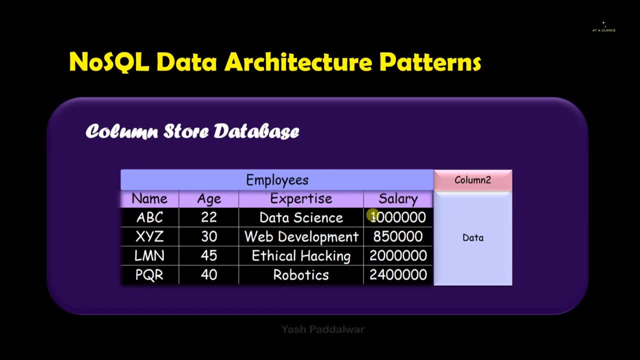 two may have several columns inside it. So let's represent this with the help of data. So now you can see that this employees and some other columns can combine together and a single column. Hence the column. company column is the super column. for all these columns, Employees is. 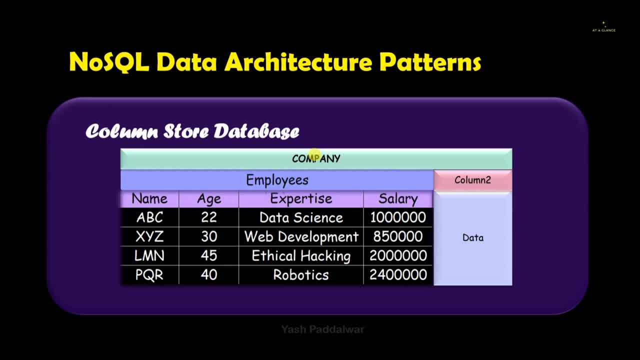 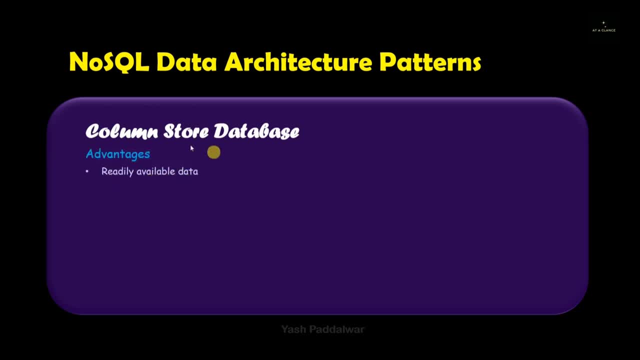 the super column for the columns name, age, expertise and salary. I hope by this example the concept of column store database is clear. Now let's have a look at the advantages. So the first advantage is that the data is readily available. This is the most important advantage. 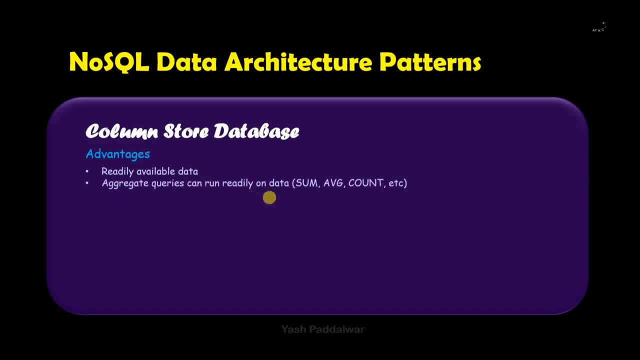 of this column store database, You can see that, like in RDBMS, we have all the data in structured form. So you can see that in RDBMS, we have all the data in structured form. So you can see that in RDBMS, we have all the data in structured format. Now, because of this, 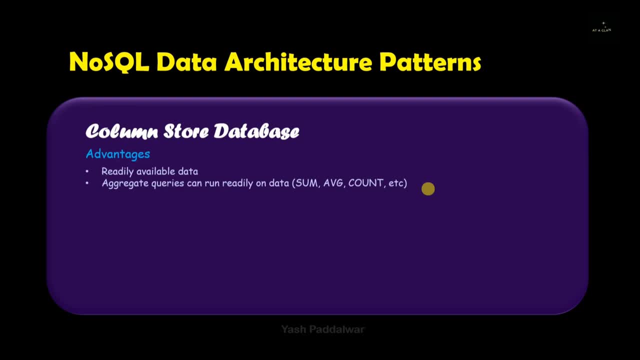 we can perform all the aggregate operations, For example, some average count, et cetera, because the data is readily available and all these operations can be easily performed over it. Now, this advantage is that it's not efficient with online transactional processing, because it 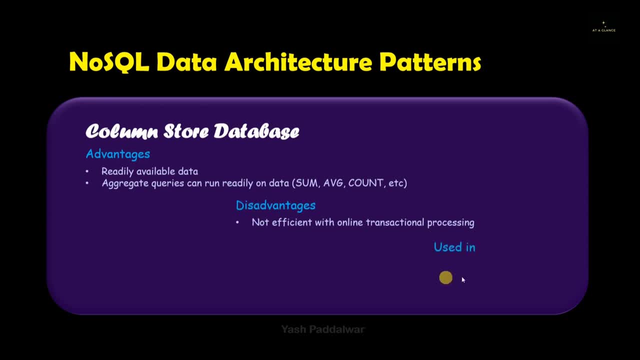 highly made and used for the online analytical processing. Hence it does not have a strong side for the OLTP operations. Now, this is highly used in the database, like HBase, which is an Apache product, And it can also be used in Cassandra. 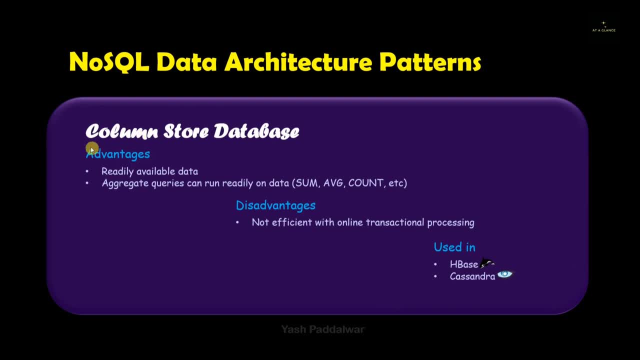 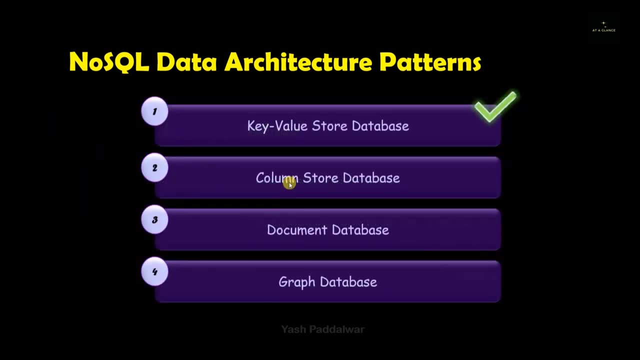 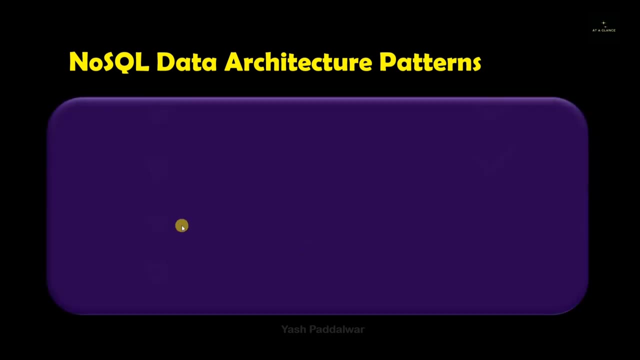 which is yet another popular database. So I hope the concept of column store database is very much clear to you all. So let's move on to the another data architecture pattern of NoSQL, which is the document database. So let's first have an overview of the document database. So basically, 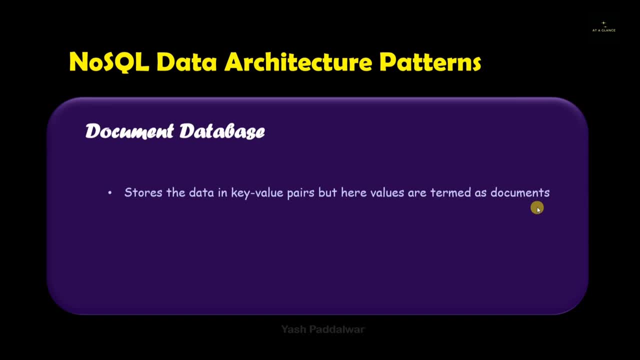 it stores the data in the form of key value pairs, but this time the value is termed as documents, which is more or less similar to semi-structured data. Now, as we have already seen, that key must be unique. Now these documents can be any complex data structure, For example arrays, strings. 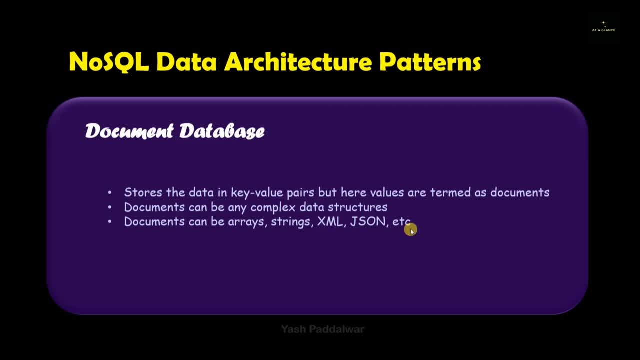 XML, which is extensible markup language, or it can be JSON, which is JavaScript object notation. So this is one thing: that documents can have nest inside it, which means multiple documents can be inside a single document, which can increase the complexity of storage of data. Now to understand. 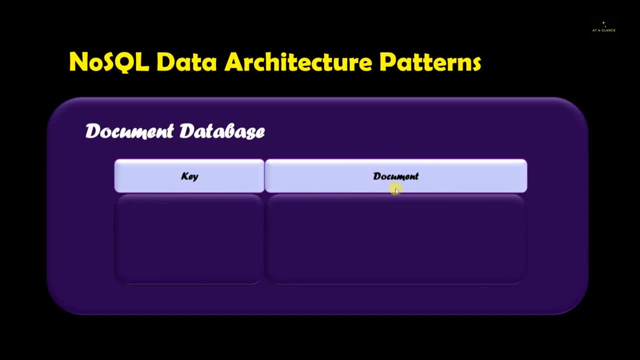 this clearly. let's see an example. So here the data is stored in two parts. First is a unique key- Let's say it is one in this case- and second is the document. Now I already said that document can be of any complex data structure. 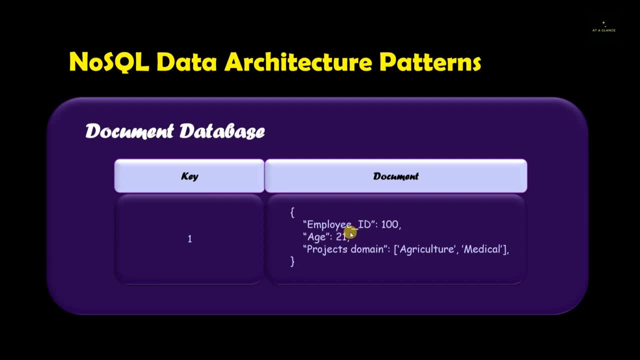 Here we have used JSON, So you can see that the data is stored in the form of key value pairs inside curly parenthesis. You can see, here we have stored the information of an employee. The first is the employee ID, The second is the age and third is the project domain. You can see. 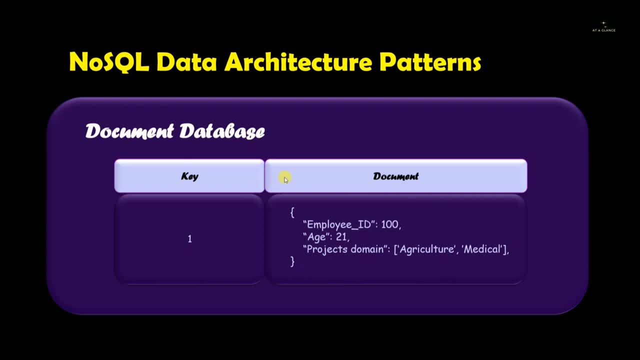 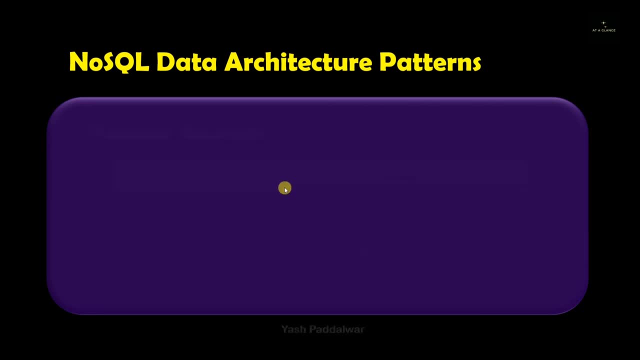 that the project domain's value is in the form of an array. The array contains two elements, As said value can be of any form of complex data structure. I hope the example is clear to you all. Now let's see the advantages of it. So first advantage is that it is useful for semi-structured 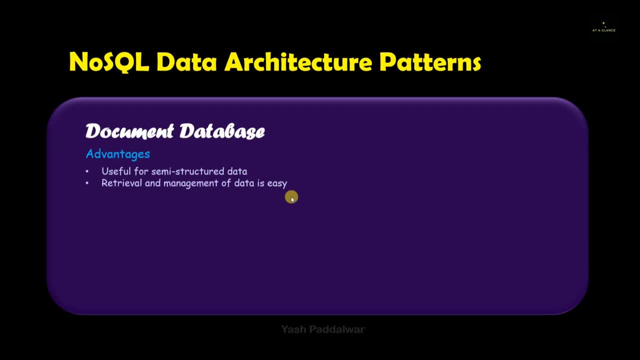 data And also using this document database, the retrieval and management becomes so easy. Now let's have a look at the disadvantage. Now you can see that the data is stored in the form of semi-structured data, So the aggregate operations may not work. 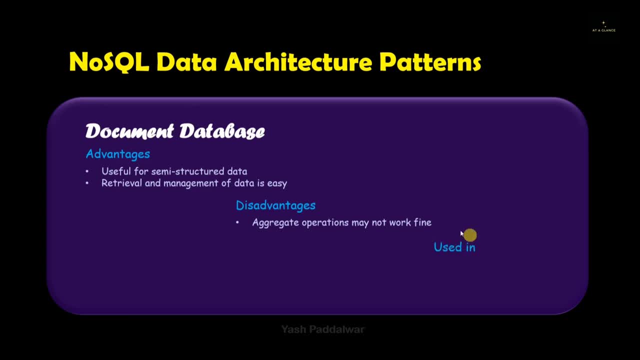 fine, or it may take a lot of time to accurately perform the aggregate operations. Now the concept about annotations: this will not be covered in this Semistructured Data migration, So all you have to do is garnish the data, clean up the code papers and actually animate the primary and secondary Savior. 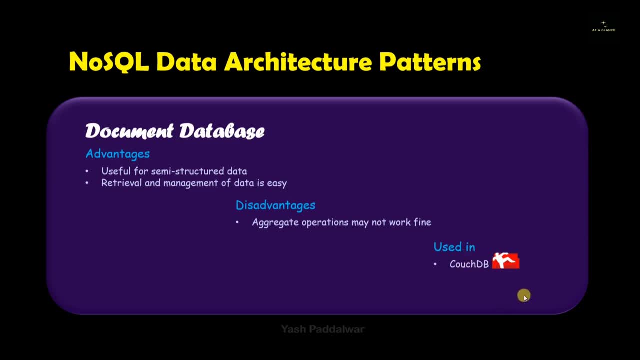 So now you can see that the OMG options are in there. However, when you do these dużo of tasks, it means that the results come with a valid data structure. Now, the concept of document database is widely used in so many databases, for example CoachDB. 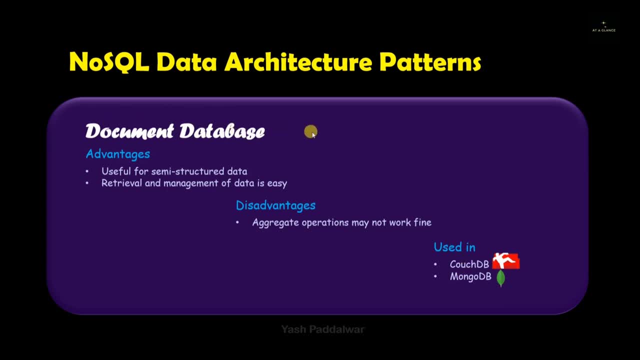 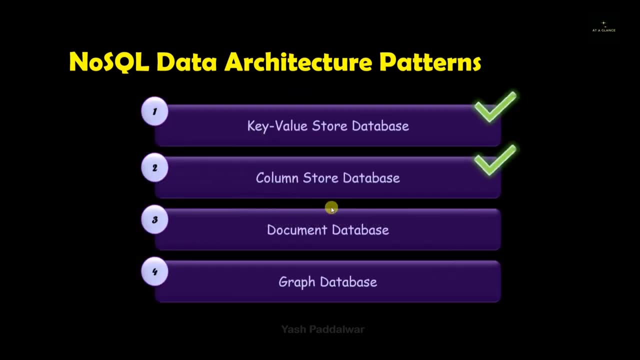 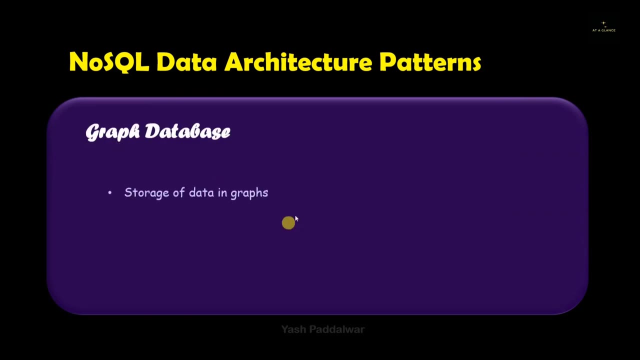 and MongoDB. You might have heard of the term MongoDB, it is so popular. So that's it about document database. Now let's move on to the last NoSQL data architecture pattern, which is graph database. So let's have an overview of the graph database. Graph database stores the data in 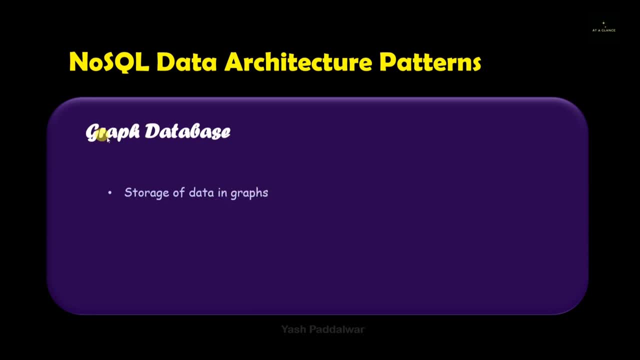 the form of graphs. You might have heard this term: graphs in data structures and algorithms. Yes, the same graph is used here. Graphs are nothing but basic data structures. that states the relationship between objects. Now, in this case, objects are called as nodes and these nodes are: 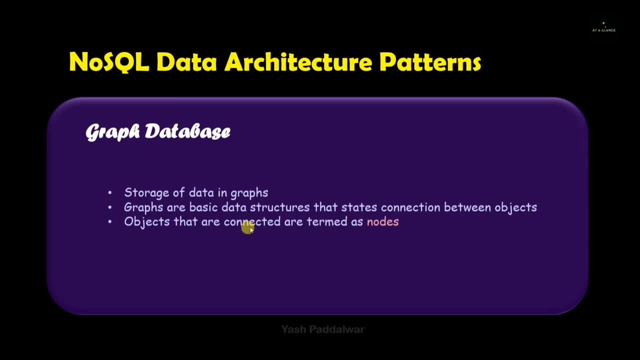 connected to every other node and the connection that is used to define the relationships between these objects. So I hope this concept is clear. Graph consists of two things: nodes and edges. Nodes are nothing but objects and they are connected to each other, and the edges are nothing but the connections. 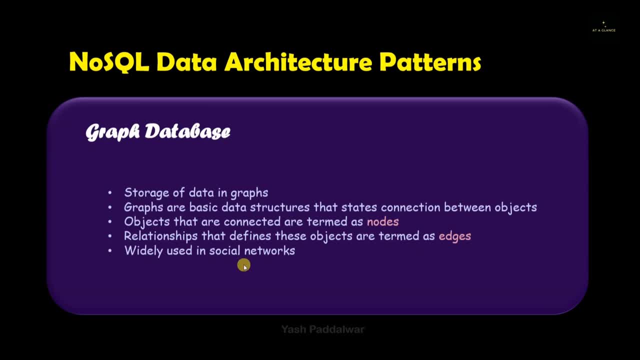 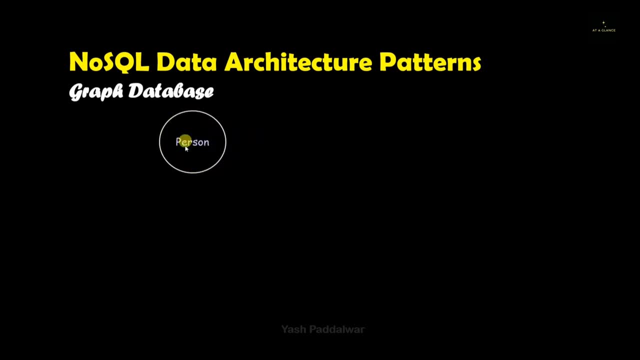 that is used to define the relationships between these nodes. Now this graph database is widely used in social network domain. So let's have a look at this graph database example. So let's say we have our first node, Which is termed as person. Similarly, let's include one more node, of person, So in all we have two. 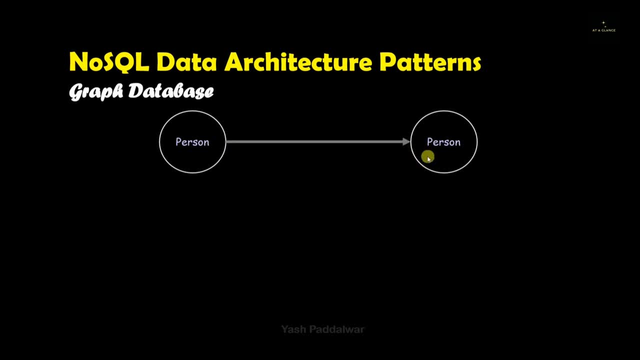 nodes of person. Now let's say, the relationship between these two nodes is defined by this edge which states the first person is the friend of the second person. So here relationship has been defined. Now let's include one more node, which is bicycle, which is connected to first person and 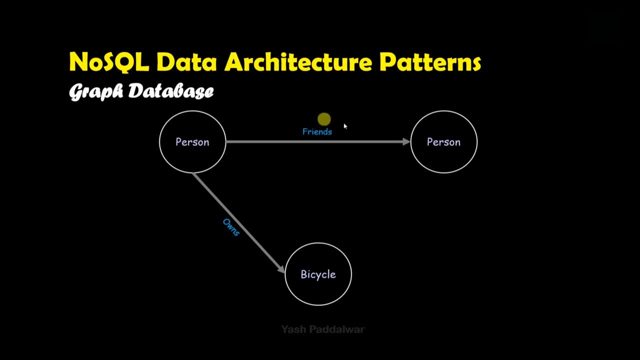 the relationship is that The person one owns this bicycle. Now let's connect the person two with the node bicycle, with the relationship that the person two is driving this bicycle. So you can see how we have established the relationship between these three nodes. Person one and person two are friends and person one owns this. 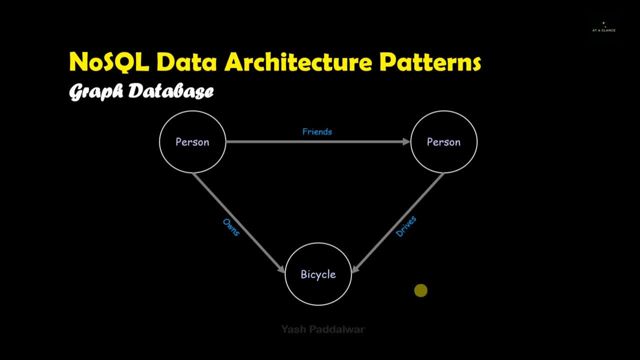 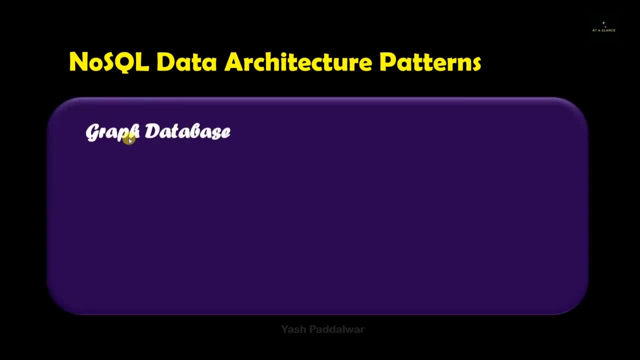 bicycle and person two is driving this bicycle. Similarly, in graph database, millions of nodes connects to each other and establish relationships and it stores information in this particular way. So let's have a look at the advantages of using this particular database. So first advantage is that it.